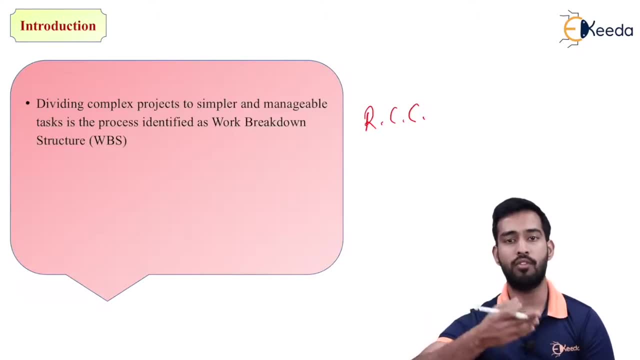 In concreting, also placing At the same time you have to go for vibration. After placing and setting of your concrete you have to go for curing work. So this RCC is also divided into different activities. So RCC we can know as an event. 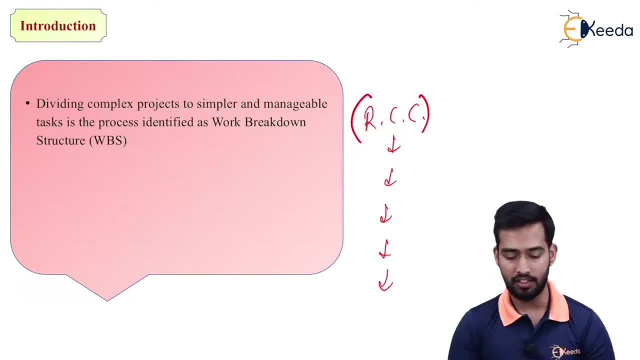 And which is divided into different activities. So that is nothing but your work breakdown structure. So usually the project managers use this method for simplifying the project execution. In WBS, much larger tasks are broken down to manageable chunks of work. 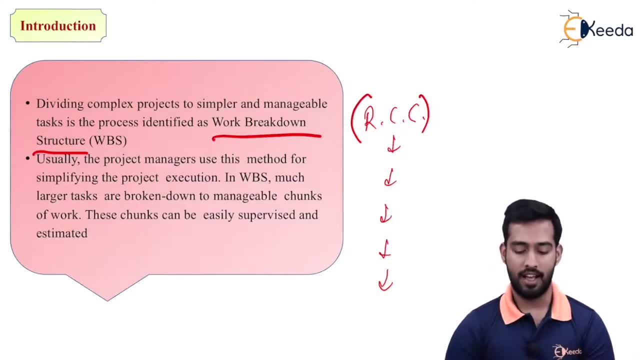 This chunk can be easily supervised and estimated If someone tells you you have to build this building. So building a building is a much complicated thing. This thing we have to divide into different activities, And these activities are then manageable within that particular time. 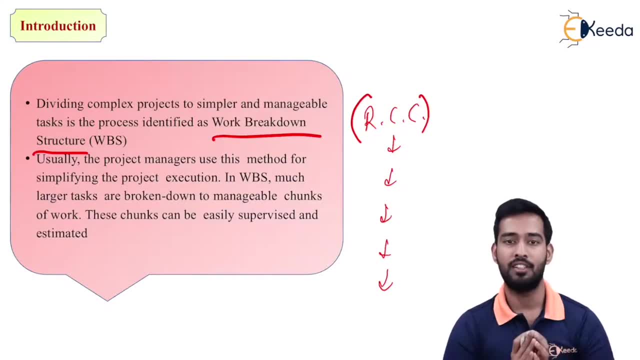 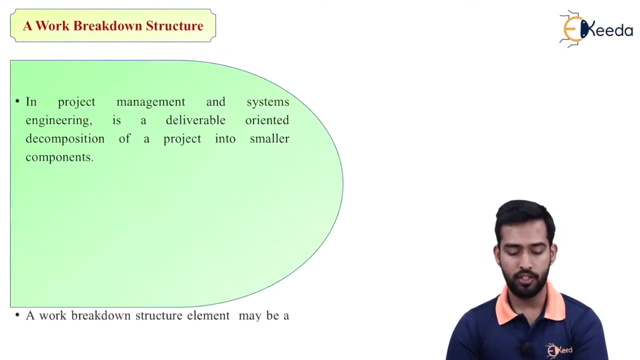 So we have to set a duration for that particular activity. If we achieve completion of these activities, then only our project will be completed in the desired time. In project management and system engineering it is a oriented decomposition of the project into smaller components. 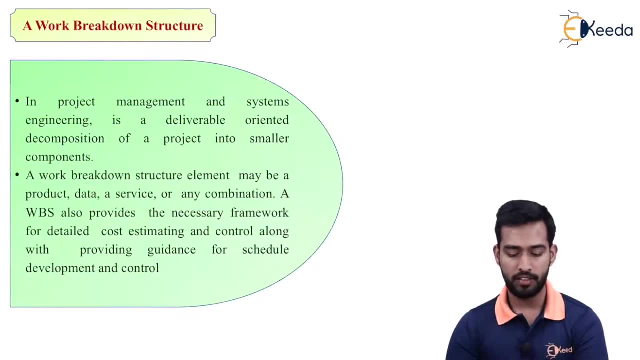 A work breakdown structure element may be product data service or any combination. WBS also provides the necessary form work for detailed cost estimating and control, Along with providing guidance for the scheduled department and control, So it also gives us more cost estimate. 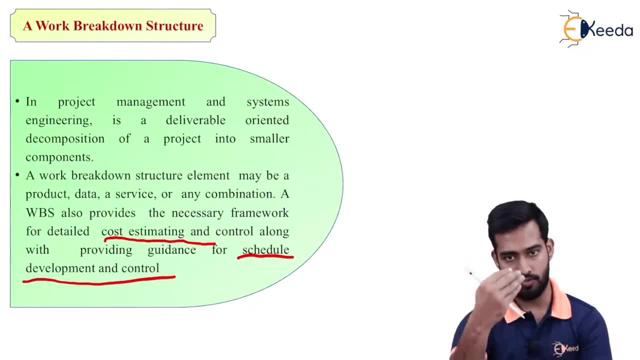 So after dividing the activities or the whole work into different activities, we can identify the cost required to complete that particular activity. So the cost estimation also can be done And at the same time it is useful for scheduling of your activities. 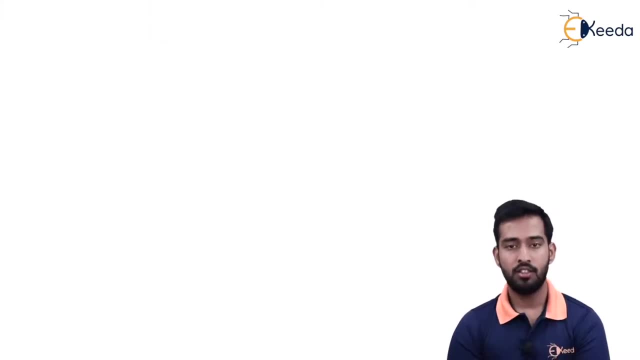 As we have seen in bar charts. So bar charts, To prepare bar chart we have to divide the work into work breakdown structure And then only we can provide the bar charts For preparation of bar chart. also, we require to divide the whole project into different activities by using your WBS. 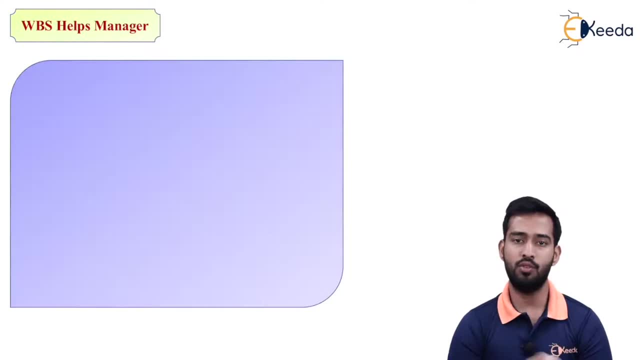 Now how it is helpful for the managers. This tool is generally useful in the managerial levels. So facilities evaluation of cost, time and technical performance of the organization on a project. Then it provides management with information appropriate to each organization level. 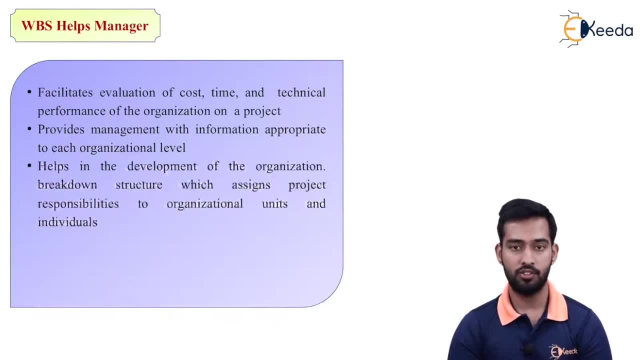 Helps in the development of the organization Breakdown the structure which assigns project responsibilities to organizational units and individuals. So, by dividing the whole project into different activities, It will give us the tool to assign the project responsibility to the particular person, For example by dividing the construction of building into different phases. 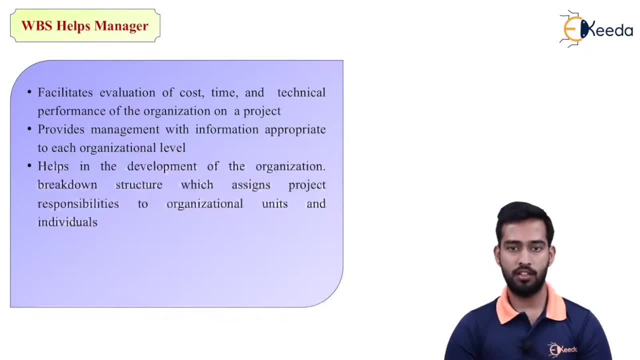 We can assign the earthwork to one person, The execution of your superstructure to one person, Then the finishing to your different contractor, So like by waterproofing, to your different contractor. So like when we divide the project into different activities will be identified. 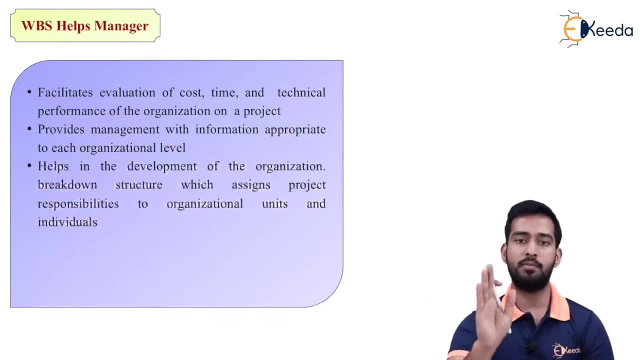 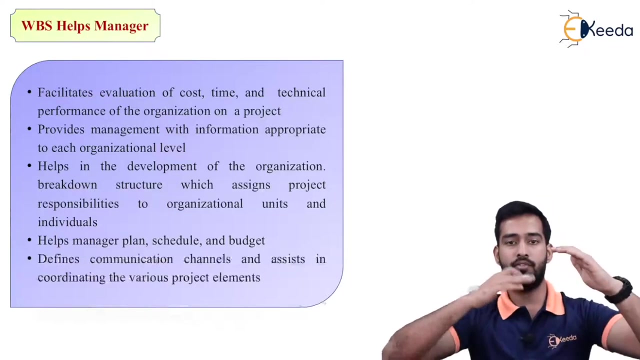 Which activity it is and will provide the expertise or a particular person who will be responsible for that particular activity. Then it helps manager to plan schedule and budget. It defines communication channels and assist in coordinating the various project elements. So at the same time, if more activities are going on, 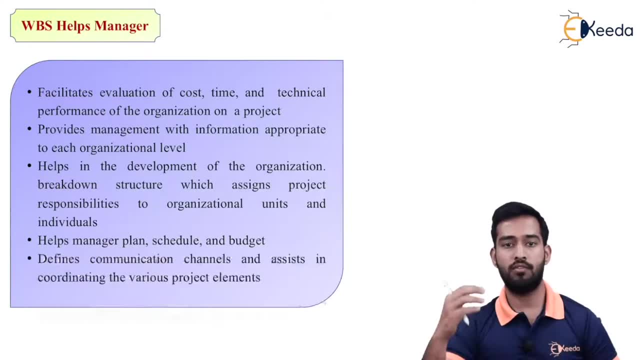 So it will give us a proper communication channel from which will give the information And it assist to coordinate with various project elements, Which activities are going on at the same time and to whom we should coordinate, Why we have to create a WBS to a particular project. 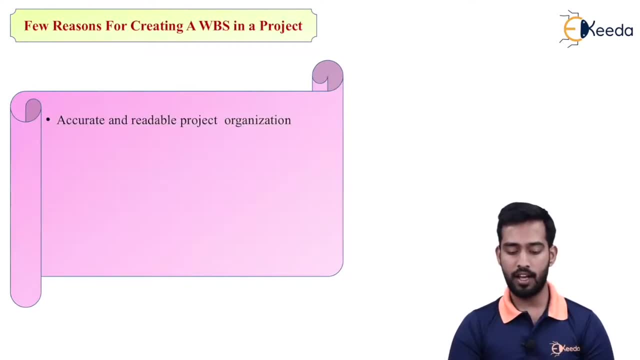 So this few reasons are there. First, accurate and ready able project organization. So this is accurate and ready, able. You can easily read what are these activities are divided. Then accurate assessment of responsibilities to the project team, So we can assign the activities or responsibilities to the project team. 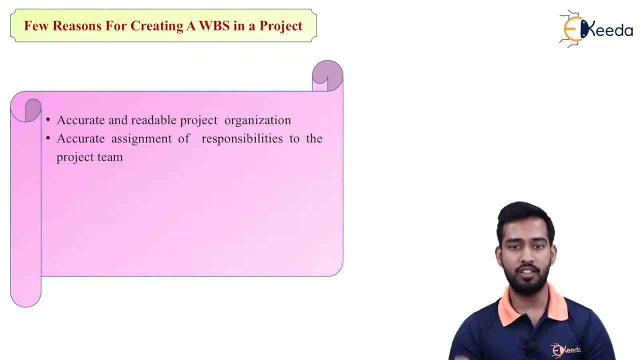 Depend upon the different activities required to perform on site. Then indicates the project milestones and control points. So, as we have discussed, If the project is to be completed within two years, So we have to set the short term goals. So the project milestones we can decide. 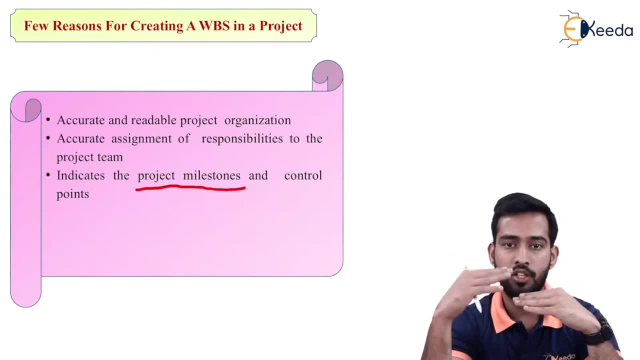 For example, within 30 days we have to reach up to first floor slab. These are milestones. So to complete this milestone, we have to observe the day to day activities, Which can be observed by using this WBS And control points. 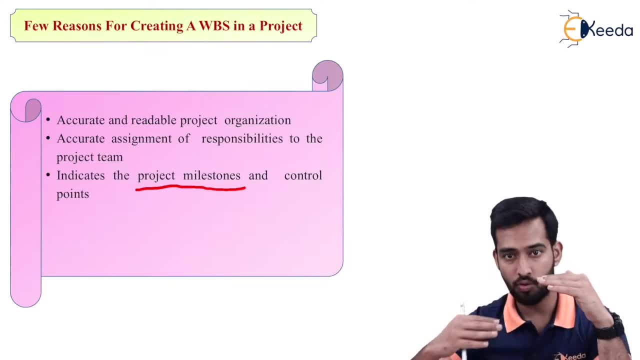 We have to set up some control points. If your project is getting slower or the project is going ahead in your schedule, Then there should be some control points on which we can control the project So that the activities coming in future will be lined up properly. 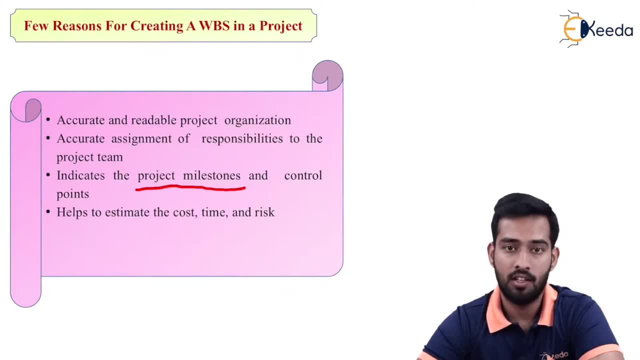 Then helps to estimate the cost, time and risk, The cost required, For example, if raw materials we have to order to complete that particular activity. So how much amount of raw material will be required for purchase of this raw material? What is the cost is required that we can identify in future only. 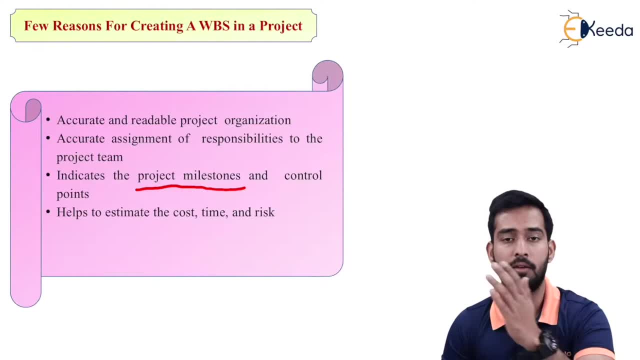 Same as the time required and the risk associated with that particular activity. Then it illustrates the project scope So the stakeholders can have a better understanding of the same. So we have to submit this to your stakeholders also, So they will easily understand what is the current scenario and what is your future plans. 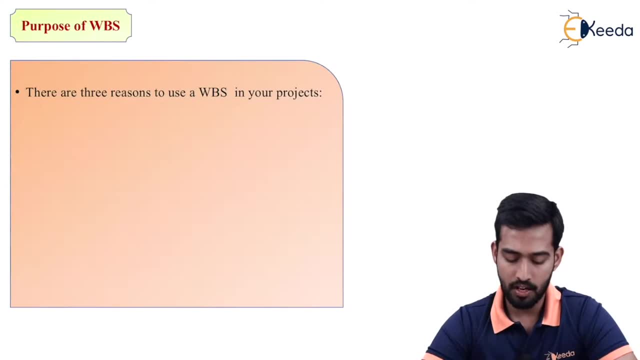 Then purpose of WBS. What is the purpose? So there are three reasons to be used WBS in your project. First is that it helps more accurately and specifically define the organization scope of your total project. So we will identify what is the scope of our project in the particular direction. 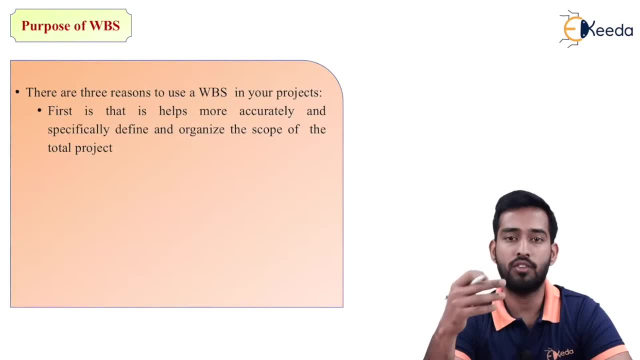 If you are constructing a residential building, What is the scope of construction? We can identify by using WBS. The second reason to use WBS in your project is to help with assigning responsibilities, then resource allocation, monitoring the project and controlling the project. 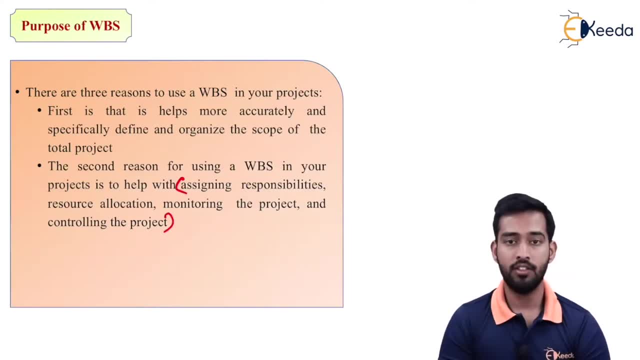 These are the main points and in which WBS is very helpful for assigning the responsibilities, As we are divided, the work, the concreting, can be assigned to a particular person or a contractor: supervisor. Then resource allocation: The number of skilled and unskilled labor required. 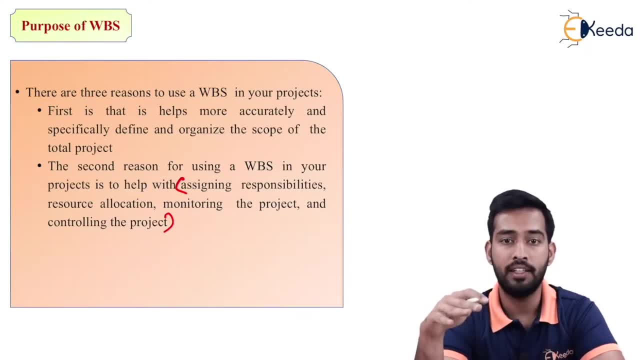 The number of equipment required for that particular activity that we can identify. Then monitoring the project. We can easily monitor what is the status of your concreting work or what is the status of your piling work, by using WBS and controlling the project. 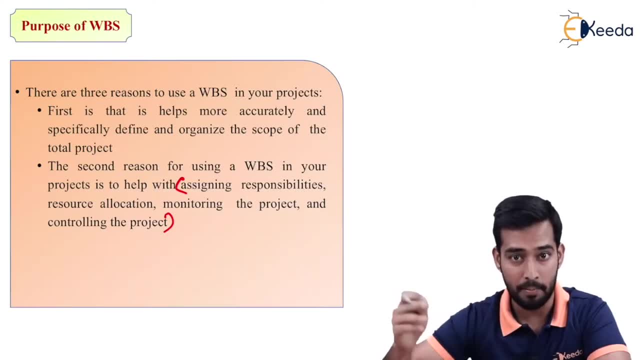 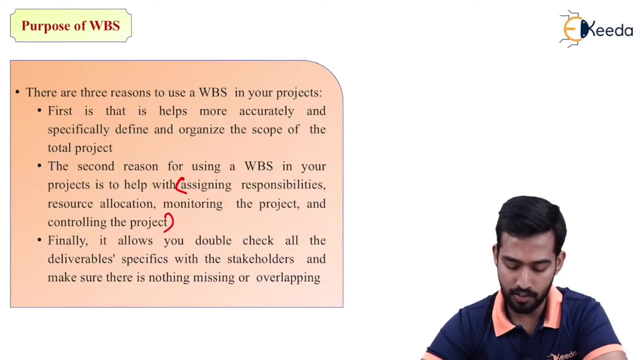 We can control the project on grid activities day by day. Finally, it allows you to double check all the data. We can check the daily variables specifics with the stakeholders and make sure there is nothing missing or overlapping. So we have given some planning to the stakeholders also before the starting of the project. 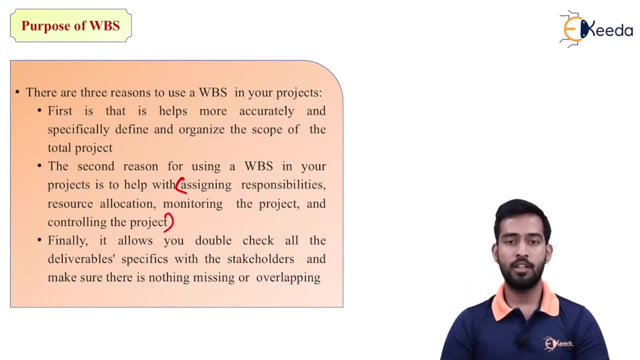 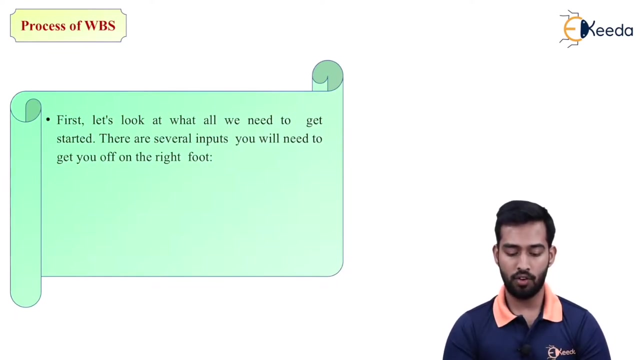 We have given them some promises, Like, for example, if we are constructing a building, we have promised our buyers that within the one month we will be completing our first slab, So we can check over it whether the objectives are achieved or not. Then the next is. there are the several inputs you will need to get you off on the right foot. 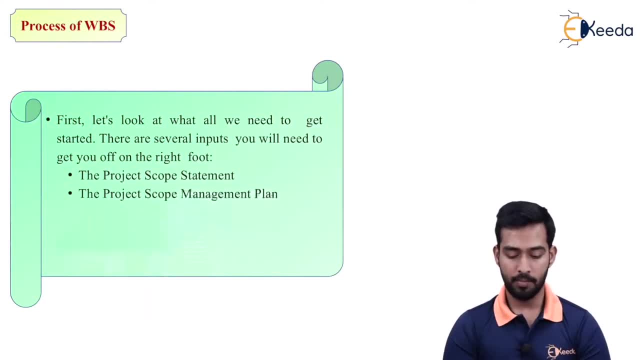 First is the project scope statement, Then the project scope management plan. Accordingly, we have to work. Then organizational process, assets: What are the assets of the organization? Then approved change request. If we have to change something, then we have to approve that request. 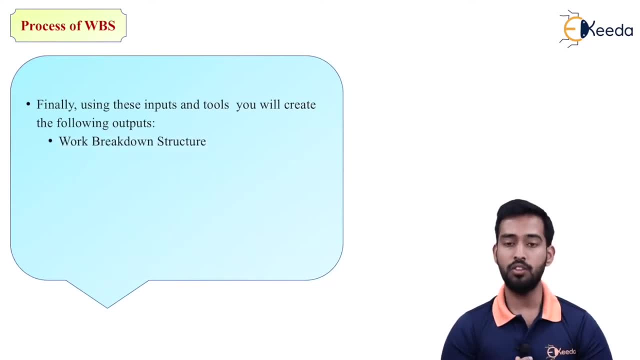 Then finally, using these inputs and tools, you will create the flowing outputs. The following outputs will be your work breakdown structure. Then we have to go with the baseline, Then project scope statement, Project scope management plans, Then requested changes. This is the process of your WBS. 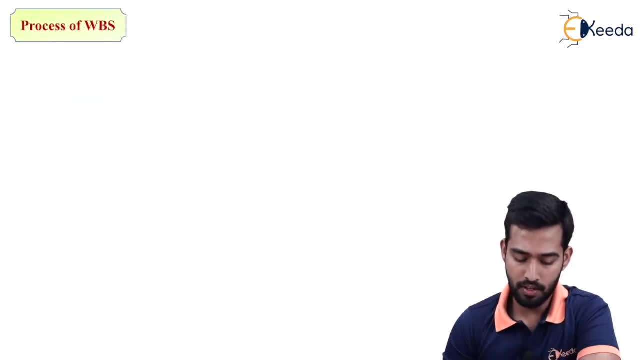 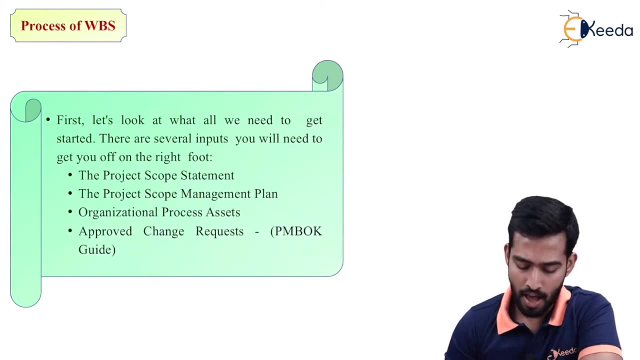 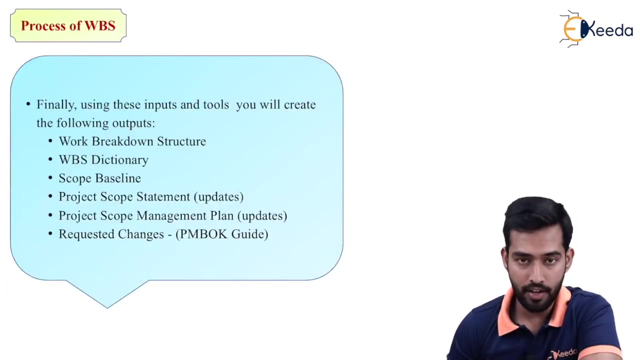 How the WBS works, The process of WBS we have discussed. In this we have to see some activities, which are the inputs. These inputs we have to see After getting the inputs. what are the outputs that we have to identify? After finding out the outputs, now construction of your WBS.